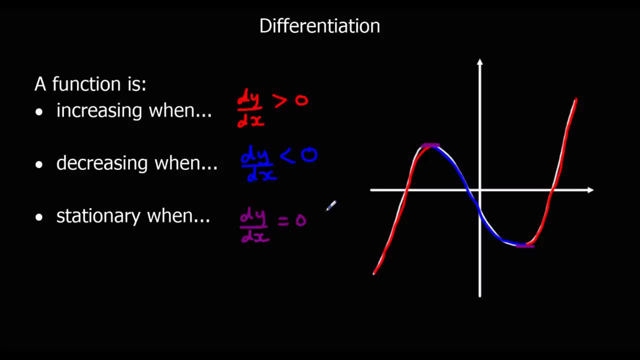 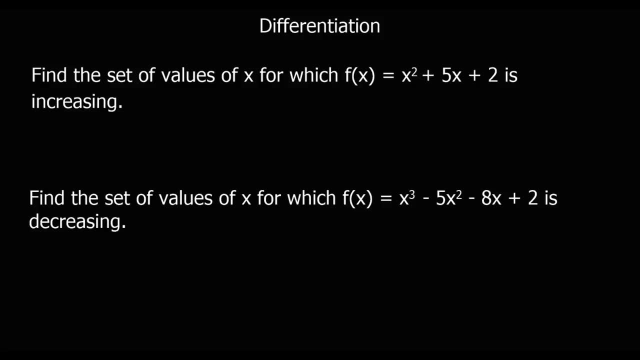 decreasing when dy x is negative and stationary where dy dx is equal to zero. okay, we've got some questions here. the first one says: find the set of values of x for which this function is increasing. so if we want to know where a function is increasing, that means dy dx. the gradient function is positive, bigger than zero, so the function is going to be. 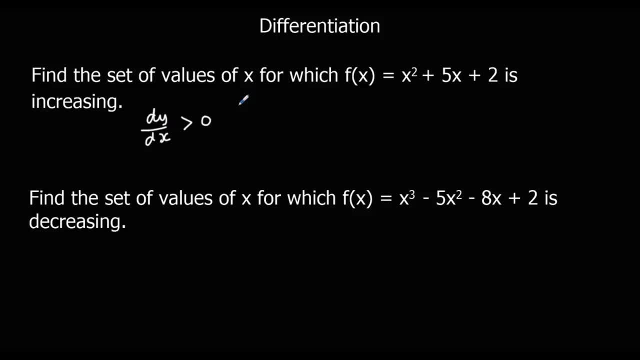 increasing when dy dx is positive. so we need to find dy dx, so we need to differentiate the function. so if i differentiate the function, i'm going to use this notation- it means exactly the same as dy dx, so the gradient function is. and then to differentiate, i'm going to times by the power. 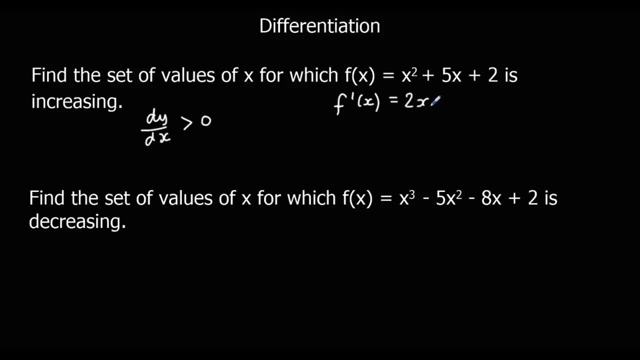 take one off the power, so that's going to be 2x plus 5. so the gradient function is 2x plus 5 and i need to know where it's increasing, where it's positive. so 2x plus 5 is positive, increasing, so it's bigger than zero. i'm going to solve this now, so i'm going to. 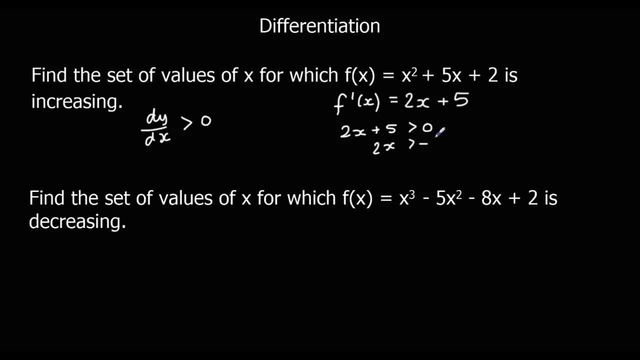 minus 5 from both sides and divide by 2. so there we have it, so the set of values of x for which the function is increasing, that's where x is bigger than minus 5 over 2 or minus 2.5. same thing for the next question, but it says: find the set of. 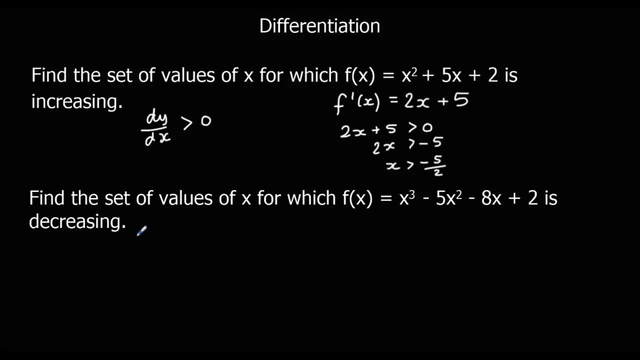 values of x for which this function is decreasing. so it's where dy dx is negative, less than zero this time. so first step, again we need to differentiate it, find the gradient function, so our dy dx, this time our f dash x. we're going to times by the power and 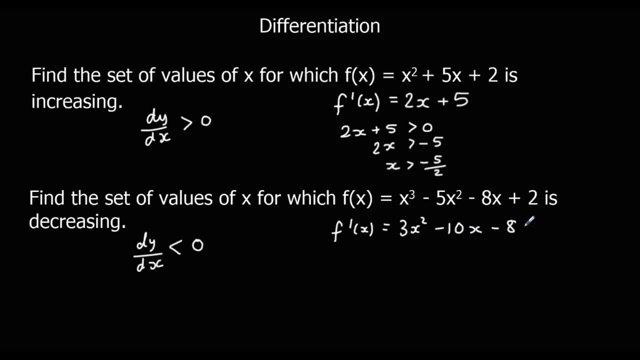 take one off the power. again same process. so we should get our differentiated function as 3x squared minus 10x minus 8. now we need to make it less than zero. so we know 3x squared minus 10x minus 8 our gradient. 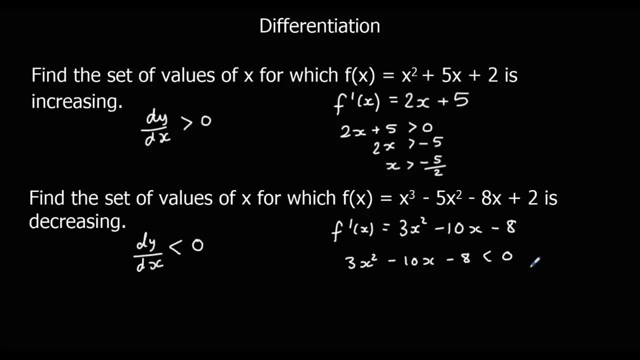 function is negative less than zero. so we've got a quadratic to solve. now the easiest way to solve it is going to be to factorize it. if it doesn't factorize, we can, of course, use the quadratic formula, but this one does factorize, so we're going to have 3x in one bracket. 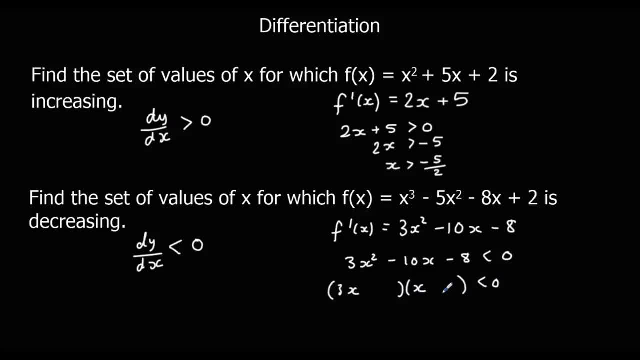 and x in the other bracket and it's going to be. that's going to give me a minus 12 plus 2 for my minus 10 and they multiply to give me the negative 8. there's lots of methods people use to factorize quadratics for coefficient of greater. 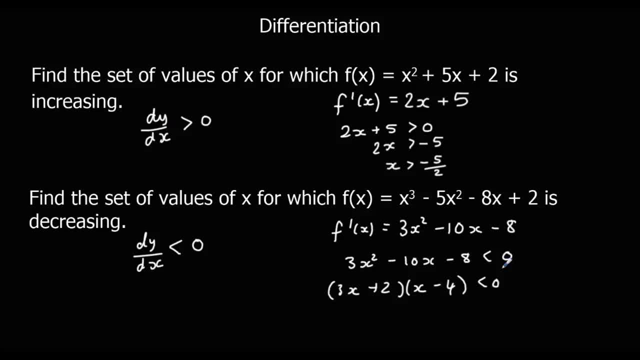 than 1 in front of the x squared. but that's the answer. she should. you should get so, and so I've got. that's it for now. Thank you for watching. x is going to cross the axes at, so it's going to cross the x-axis. that, if it. 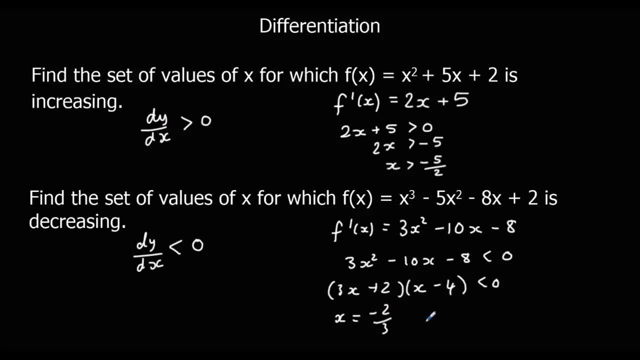 said equal 0, the solutions would be minus 2 thirds and 4. so that's where it crosses the axes. so if I give you a little sketch here, it's crossing at minus 2 thirds and at 4. so it looks something like that and we want to know. 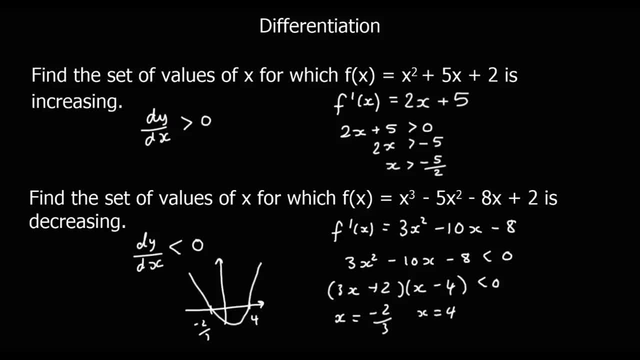 where it's less than 0. so where is it underneath the curve? where's it underneath the axis? it's this bit here. that's where it's less than 0. what are the X values here? well, we've got in between minus 2 thirds and 4, so it can. 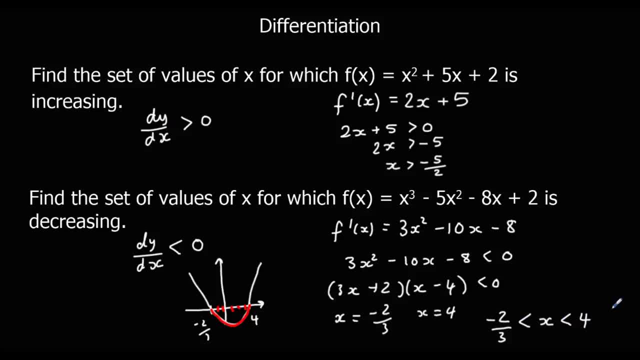 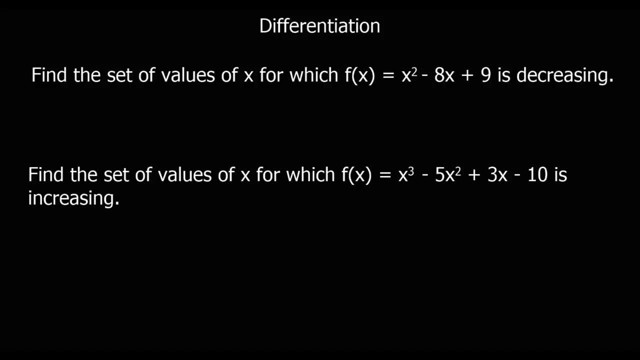 be in between minus 2 thirds and 4, and they are the set of values for which the function is decreasing. okay, here's another two questions. pause the video, give them a go, then I'll go through the answers after. okay, the first one: find the set of values of X for. 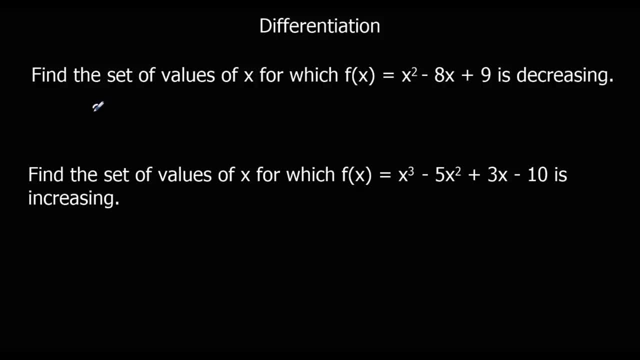 which the function is decreasing. so the function is decreasing. dy dx is negative, less than 0. so we need to find the gradient function, find dy dx first. so the gradient function is times by the power. take one off the power, remember 2x minus 8 we should get. we need to know where it's.